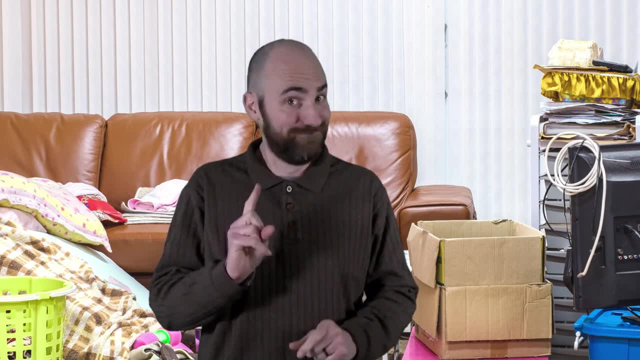 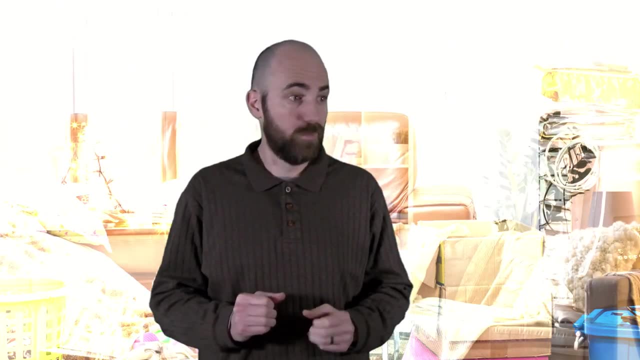 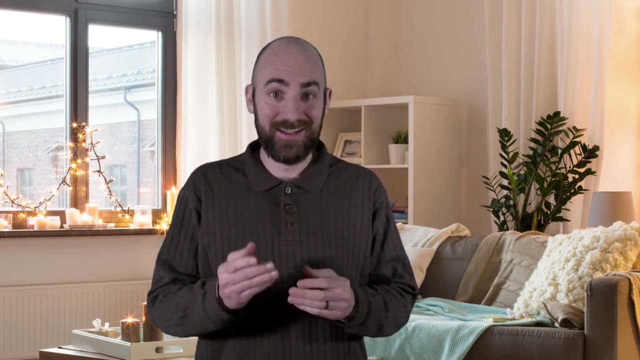 means Jesse will not need anyone else's help to complete a task. He wants to be able to turn his living room from this to this all by himself. If you feel the same way, you're in the right place. Follow along with Jesse as he learns how to take care of himself. 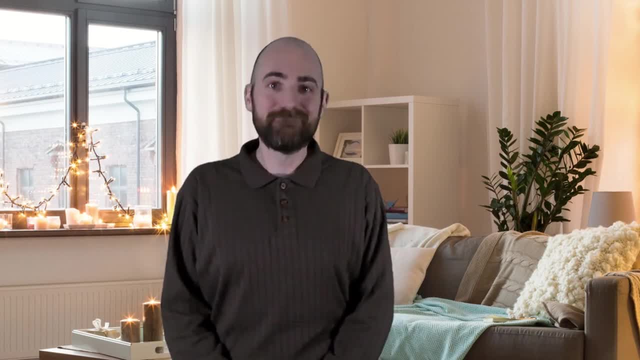 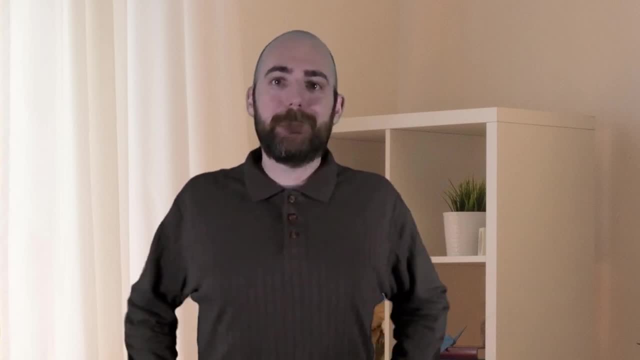 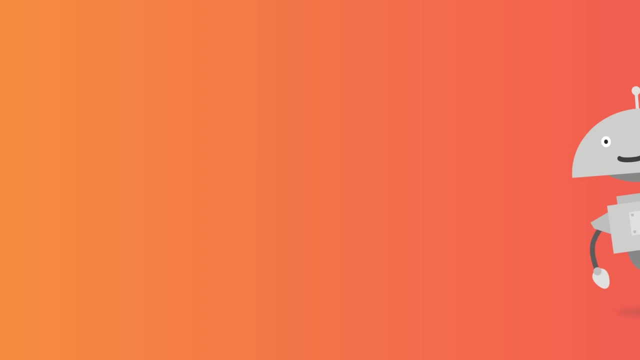 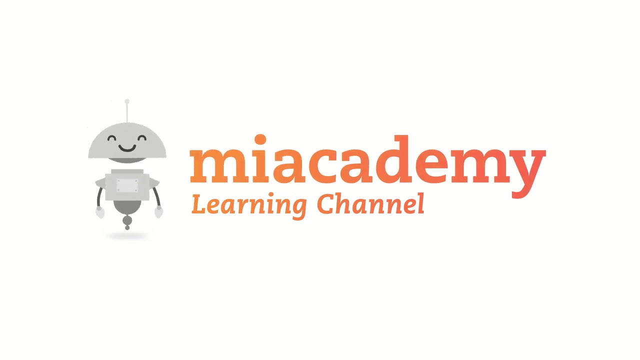 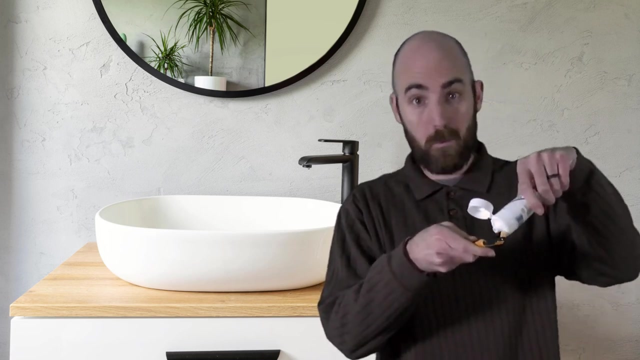 and his home. step by step. Throughout this course, you and Jesse will learn skills that will help you both grow into confident and independent members of your homes. You'll be a super helper in no time. We will explore daily tasks that are important for our health, like brushing our teeth and washing. 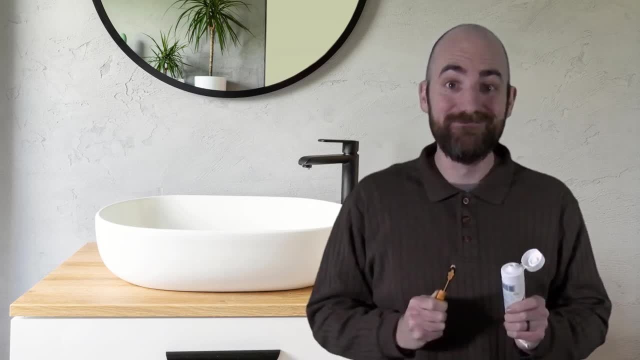 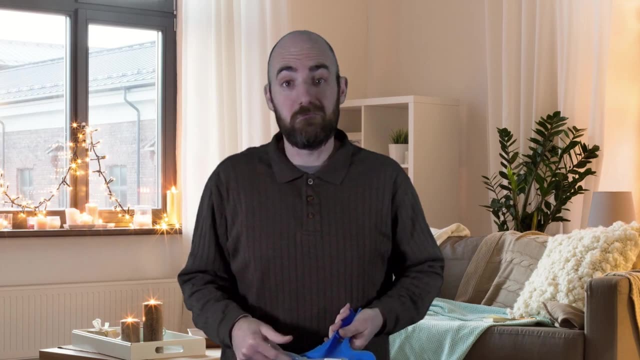 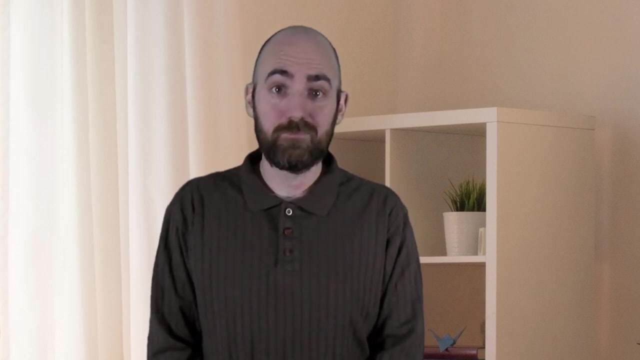 our hands. You will also learn about household chores. I know I know boring, but someone's got to do it. Helping with chores is a great way to make the adults in your life very happy and, who knows, maybe they'll even have more time to do fun things with you. 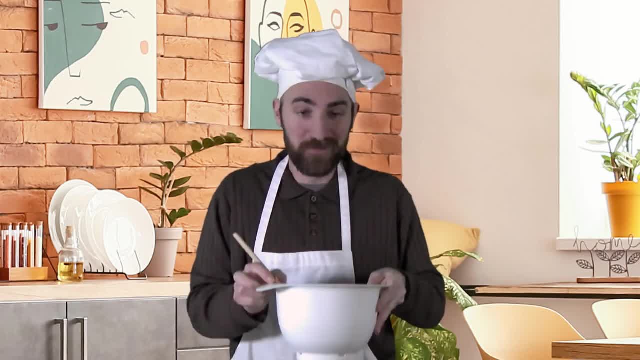 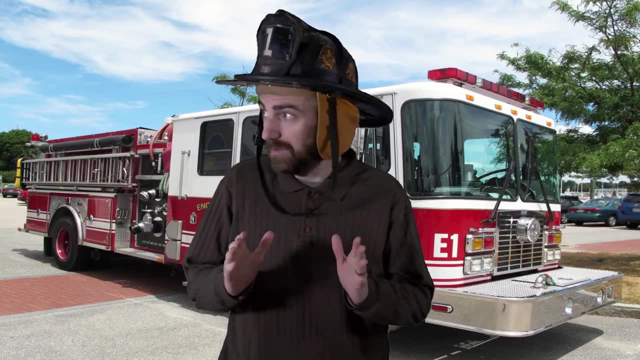 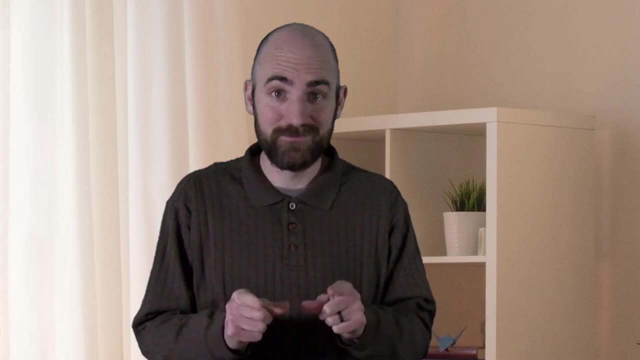 What do you think about helping in the kitchen? We will learn how to make some yummy meals. Maybe you can cook dinner sometime. And we will learn all about what to do in an emergency too. Together with Jesse, you'll learn how to problem solve and figure out the steps to. 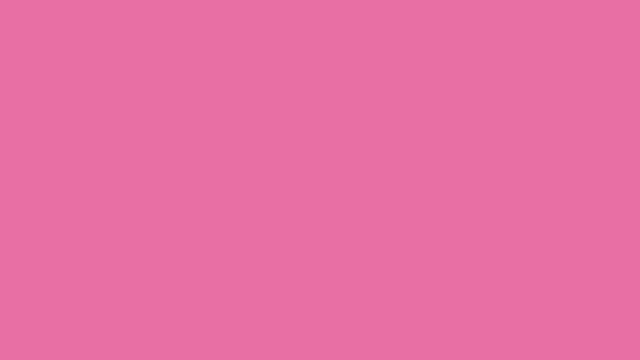 work through when you're faced with a new task. at home, We will learn where to start a task and practice working through each step together. We use the word first, next then and finally. when we talk about different steps in a process, These words can help. 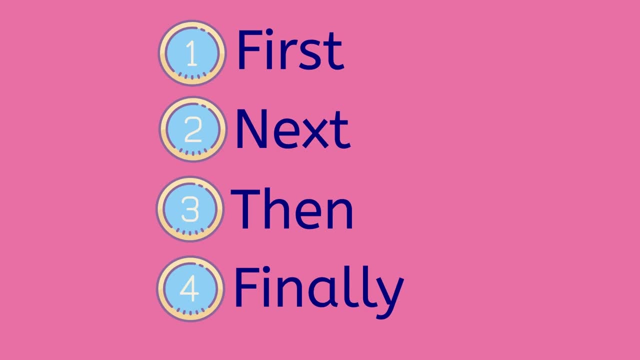 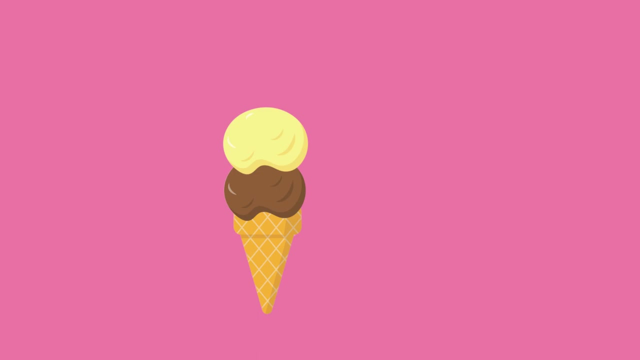 us remember what order the steps go in. For example, if we want to make an ice cream cone, what will we need to do? first, That's right, we need a cone. Then we'll add our ice cream scoops. Next, let's add some chocolate syrup. Finally, we can top it with a cherry.